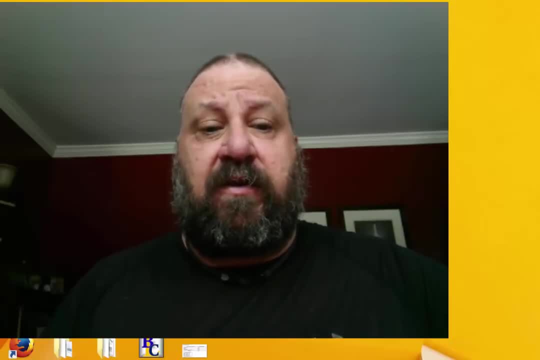 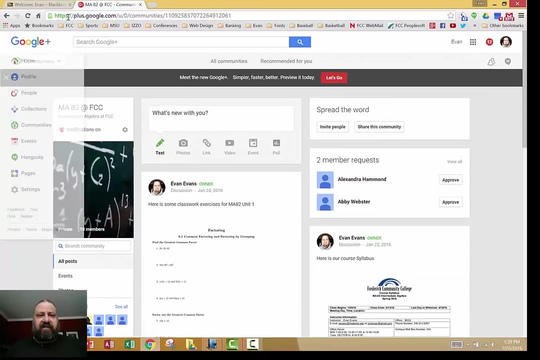 Hi, I'm Evan Evans. I'm here to walk you through how to calculate your final grade using a weighted grade system. First of all, you've got to refer to your syllabus. Most syllabus can be found either on your Blackboard page, either on the course materials or syllabus. 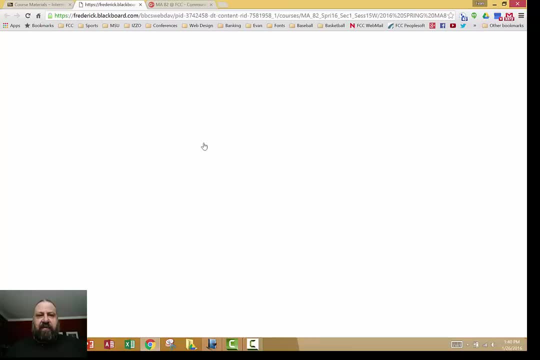 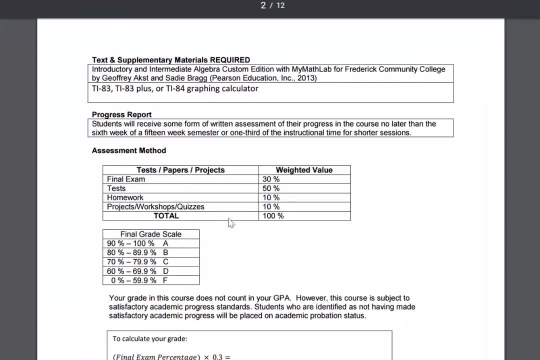 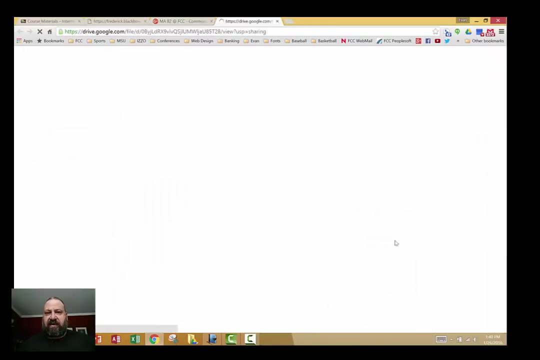 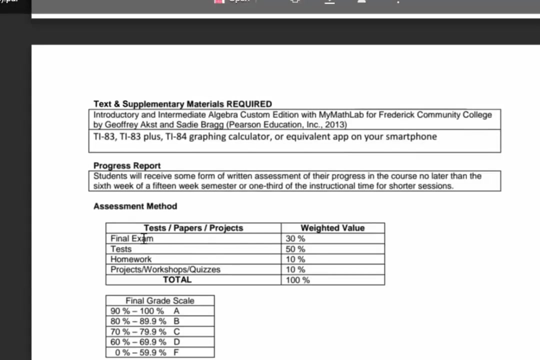 And once you download the syllabus, you want to pan on down to find out where your assessment has been. Other places you can look for it, sometimes on your Google community. a lot of times professors are posted there as well And something to click on to get the access there. So what we're interested in is calculating your final grade. So here it says: final exam is worth 30% of your overall grade. 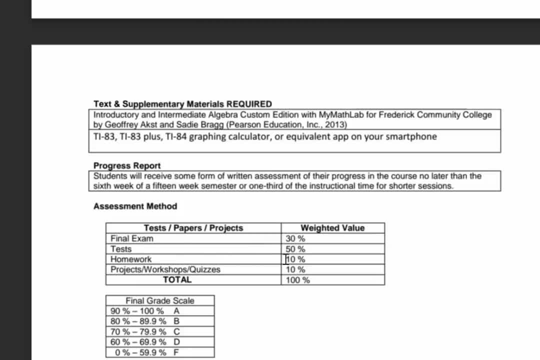 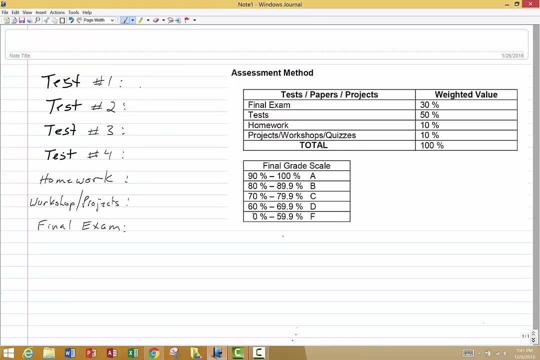 Tests- all tests- are worth 50%. Homework- Homework is worth 10%. Projects, workshops and quizzes are worth 10% as well. So this creates an area to find out how to calculate your final grade. Alright, so let's say for this particular course, on your first test you earned a 95 out of 100.. 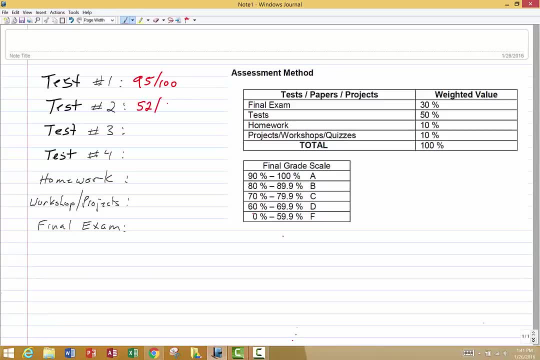 On the second test, you earned a 52 out of 65.. On the third test, you earned a 35 out of 50.. On the fourth test, you earned a 72 out of 75.. On your homework, you completed 697 problems out of a total of 820 of them. 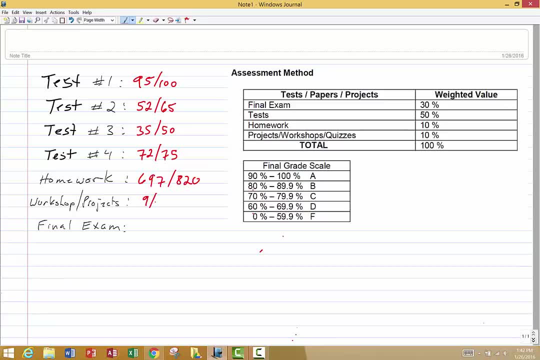 And on your workshop and projects, you earned a score of 9 out of 10.. And for your final exam, you scored a 117 out of 150.. So what we need to do is calculate the final grade. So the first thing we need to do is we need to find out what these are equivalent to in percentages. 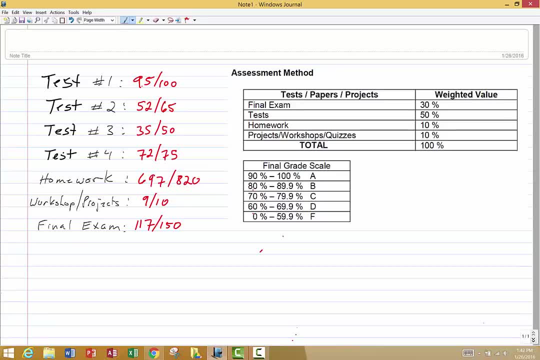 And that is simply done. You take the score divided by the total amount of points you could earn, And that looks like this: Obviously, a 95 out of 100 is a 95.. 52 out of 52 divided by 65 is equivalent to a .8 or 80%. 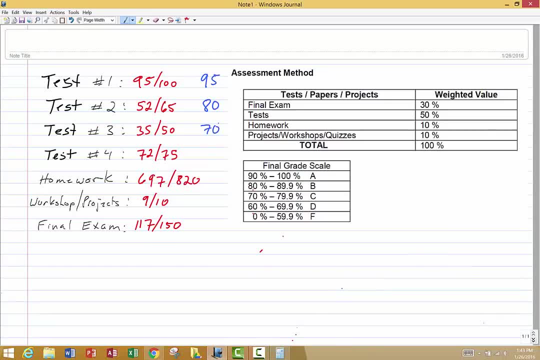 35 divided by 50 is equivalent to around 70%. 72 divided by 75 is equivalent to a 96.. All done, 697 divided by 820 possible homework problems is equivalent to an 85.. 9 out of 10 is equivalent to a 90.. 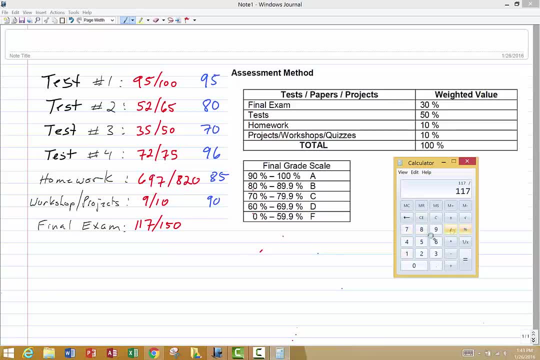 And 117 divided by 150.. 8 out of 10 is equivalent to a 78%. All right, So now that we've found the percentage of each grade that these totals are worth, now we need to have their weights And, as you look, if you look at all four tests, here are my four test scores: 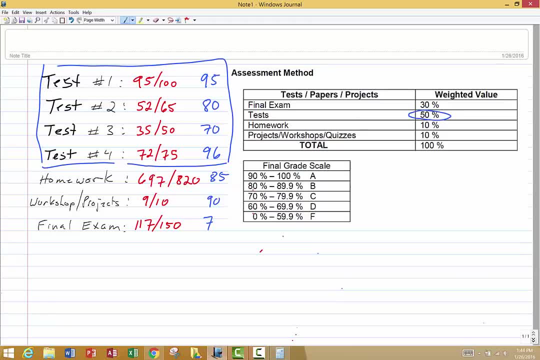 it tells me that my test scores are equivalent to 50% of my overall grade. Since there's four of them and they're equally weighted, then I need to divide that 50% by 4, which comes out to 12.5.. 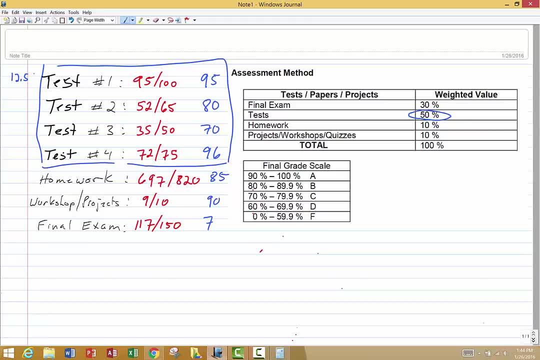 Which means each test is worth 12.5% of my overall grade: 12.5%, 12.5% and 12.5%. So, despite the fact that they have different totals, is that you don't go by the running total? 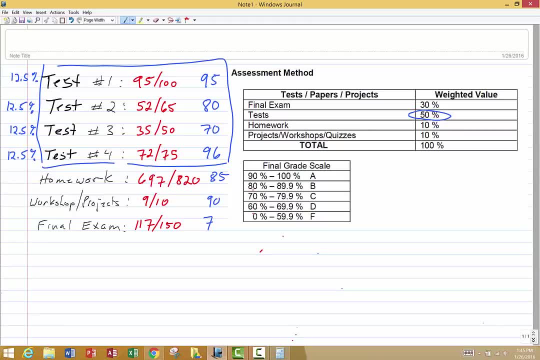 This test first, test number one, was worth 12.5% of the grade and test number two also 12.5% of my overall grade. Now you notice they're out of different points. That's why we want to stay away from the running total. 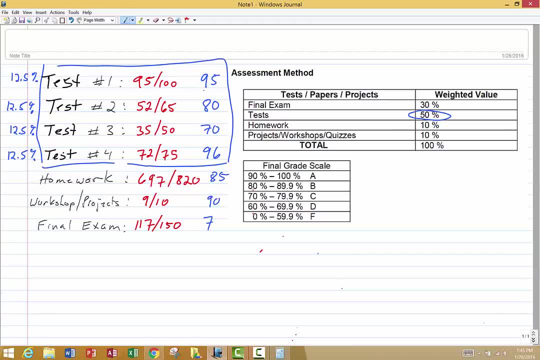 Find out the percentage they have and then find out the percentage of the overall grade Homework. it tells me that homework is worth 10% of my overall grade, so I'm going to take that score. That's worth 10% of my overall grade. 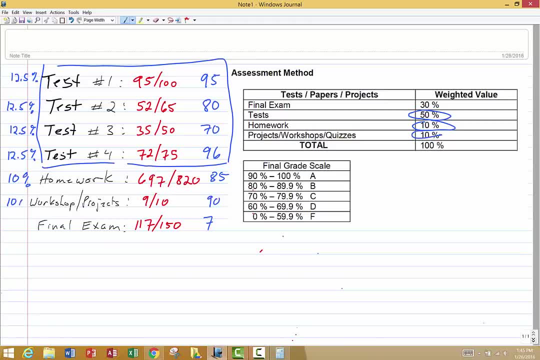 And workshops are also 10% of my overall grade, And then my final exam is 30% of my overall grade. So I have the weights over here. Here are my weights, Here are my totals. So now what I need to do is be able to calculate how to find them out. 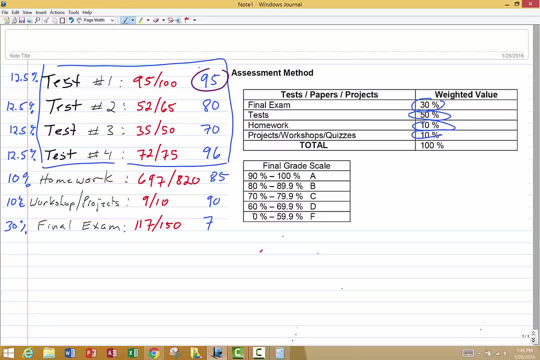 So what I do to find out my total grade is I'm going to take the amount earned, the percentage which was 95% in the first exam, and that's worth 12.5% of my overall grade. So I'll take that and multiply it by .125,. 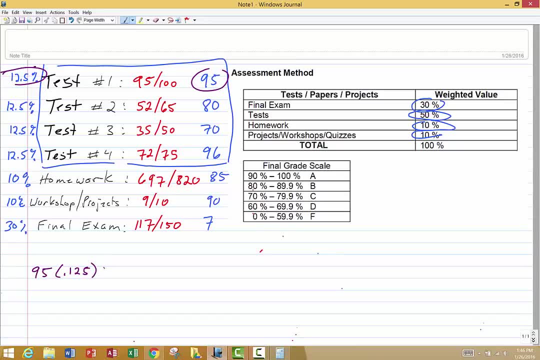 because that's 12.5% as a decimal, And then I'm going to add it to my second score of an 80,, which is also worth 12.5% of my overall grade. Add it to the 70. Times the .125.. 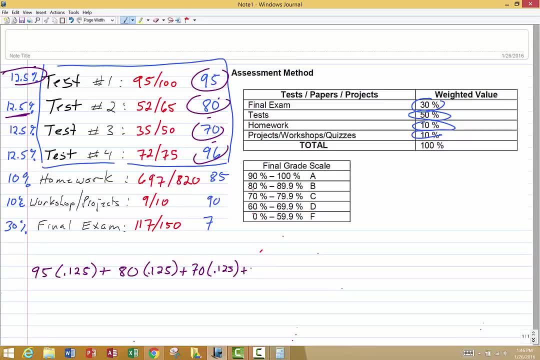 Because that's what it's worth. Then 96. Times the .125.. And now for the homework grade, I get a score of an 85. An 85. And that's worth 10% of my overall grade. so that's going to be worth .10.. 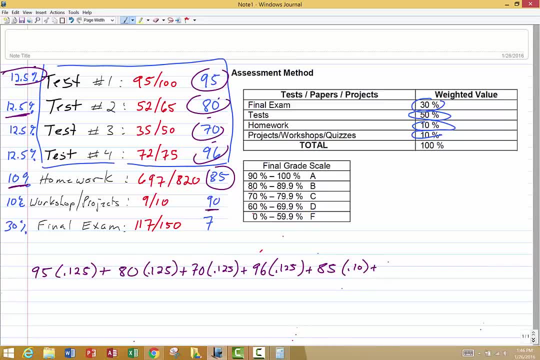 And my 90 here for my projects and homework- or, I'm sorry, projects and workshops- 90 times .10.. And then my final exam. now for my final exam. it's worth. it was a 78,, so 78 times my 30%. 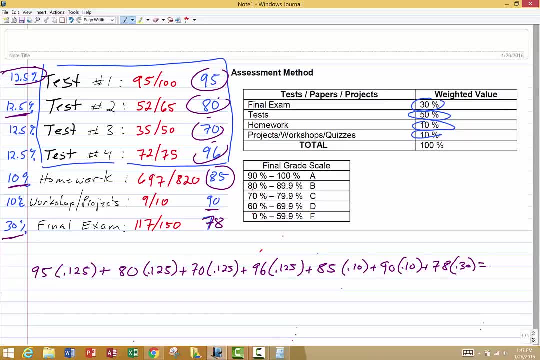 .30.. And when I add all those together it comes out to being an 83.525.. So that's going to an 83.5% Or a B. So you end up with a B for the final course. Now let's find out how we can calculate our grade. 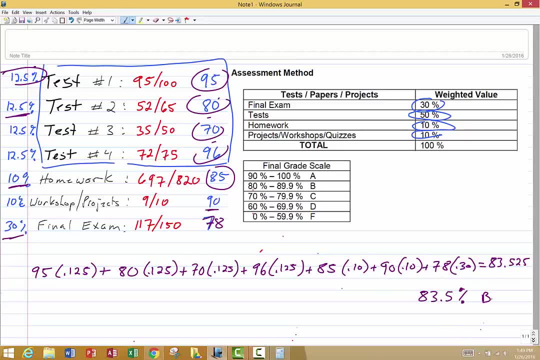 going into the final, not knowing our final grade, to try to get the desired grade we want. Let's say, going into the final exam. you have the same test scores: test one, two, three, four, same homework grade and same workshop project grade. 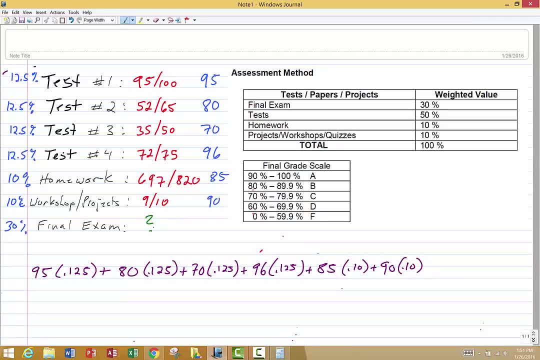 And you want to know what you need to get on the final exam in order to secure your desired grade of a B. Well, B means you need at least an 80%, So our goal right here is to get down to an 80%. 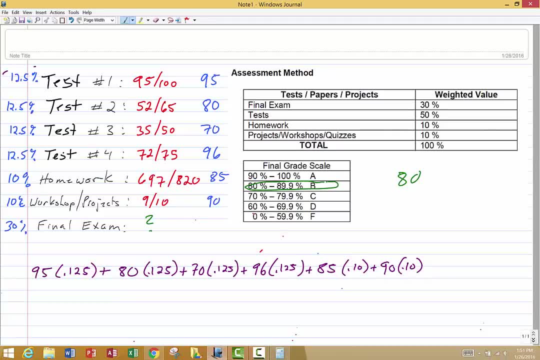 So what happens is, because this is unknown, this is going to be my X And it's still worth 30%. so it's going to be X times .30.. So what happens? I replace the last test, the first. all the other scores remain the same. 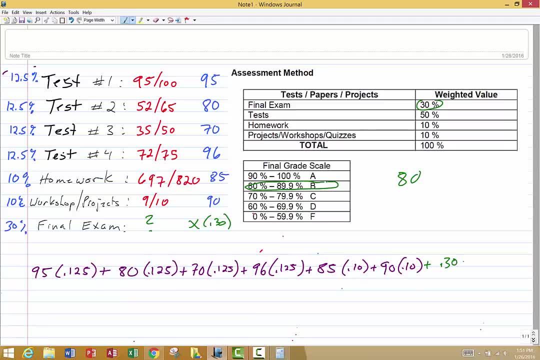 but now for my final exam. it's going to be .30 times X And it's going to be equivalent to the grade that I want to finish off with. I want to finish off with an 80. So I want to calculate with that being 80,.